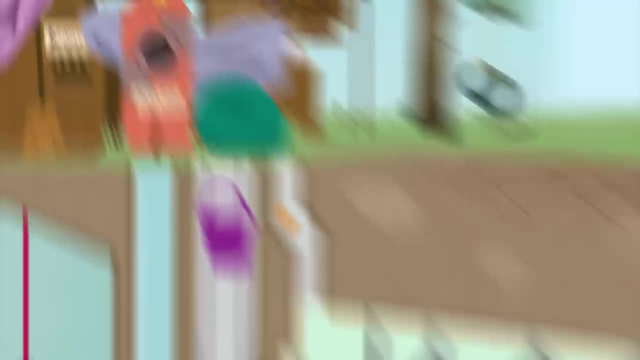 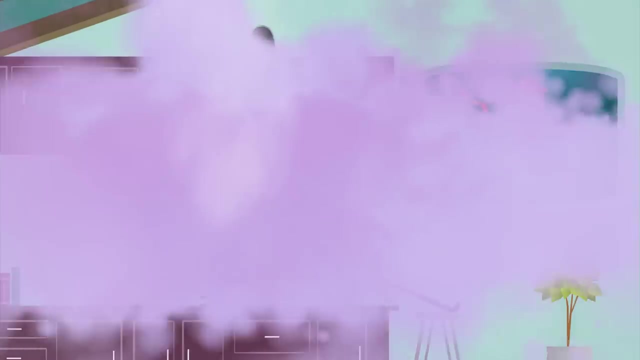 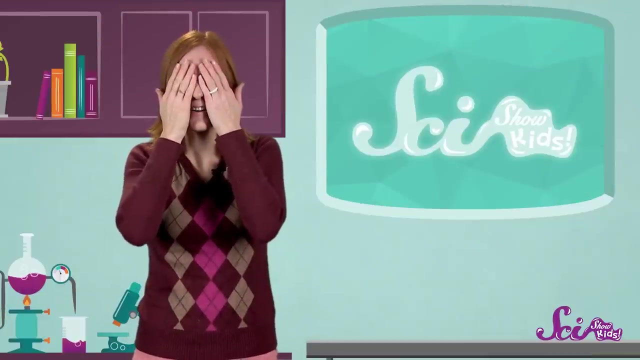 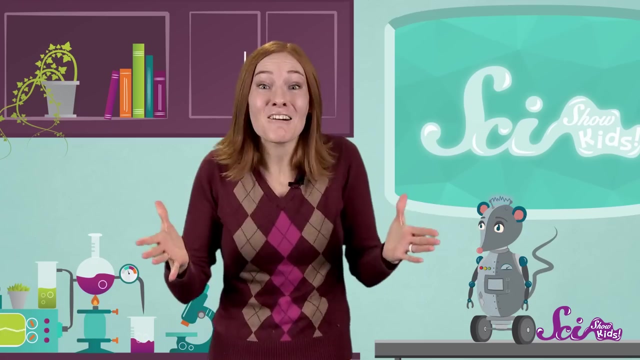 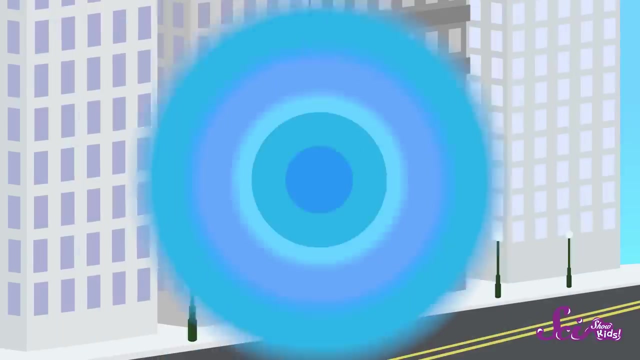 Cover your eyes for a moment and just listen. What do you hear? I hear my chemistry set bubbling and squeaks. Is that you? Sounds are all around us all the time. There are so many of them and we call sounds by a lot of different names, Like if a sound is really loud and kind of unpleasant. 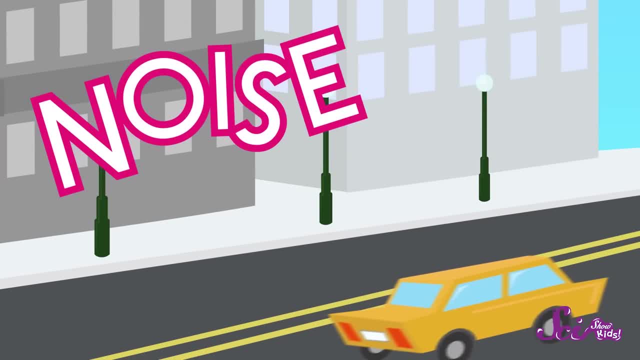 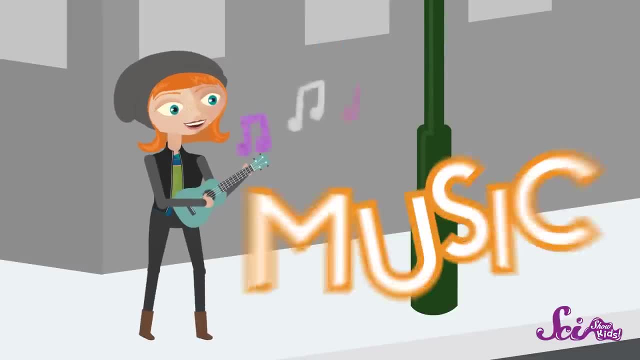 like when there's a lot of traffic going by, we sometimes call it noise, And if a sound is made by an instrument like a piano or a ukulele, we call it a note, and we call lots of notes together. music And some words are kind of like the sounds themselves, like when fireworks go boom. 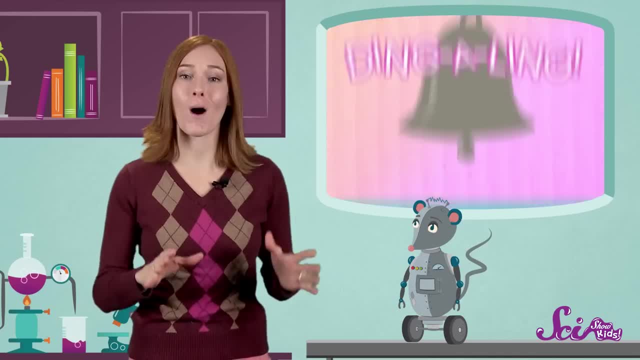 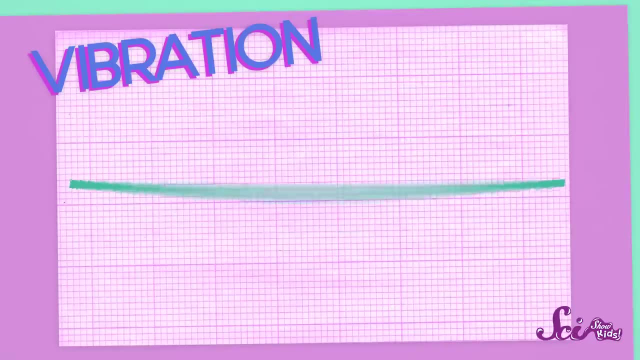 popcorn pops and bells go ding-a-ling. It doesn't matter what makes a sound, though All sounds are made the same way: through vibrations. When something vibrates, it moves back and forth really fast, So fast, in fact, that our eyes often 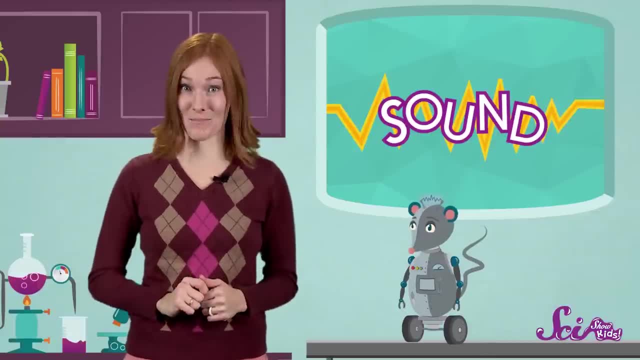 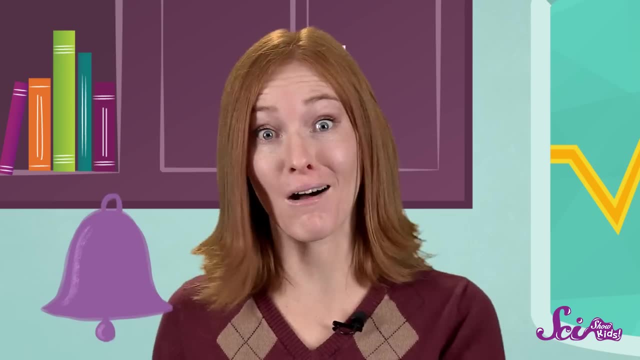 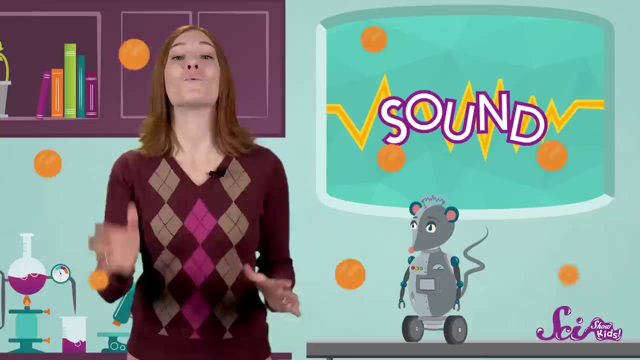 can't see it moving. But other parts of our body can sense vibrations, and I bet you know what parts those are. That's right, our ears. So how does sound get from, say a bell, to our ears? The air all around us is made of tiny particles, and these particles are what carry sound. We can. 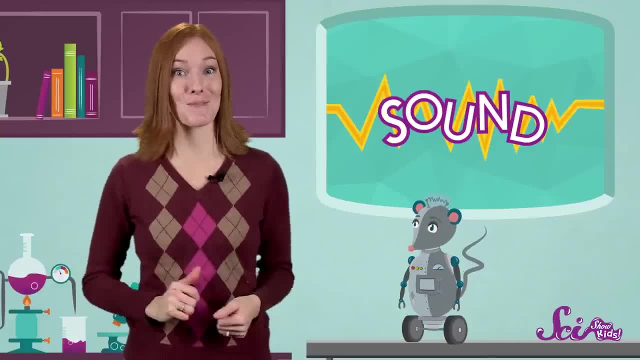 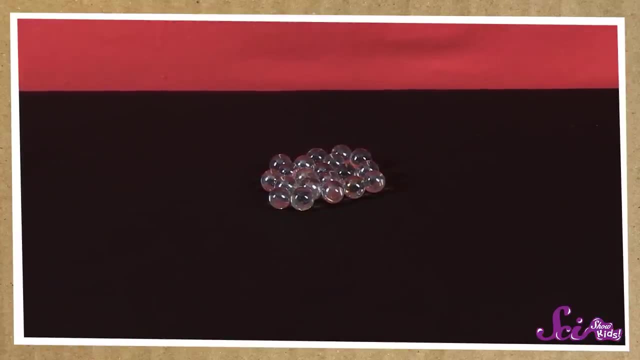 use marbles to demonstrate the teeny, tiny particles that make up the air. Let's see how, If we put a few marbles together so they're touching, then roll another marble so that it crashes into them, the group of marbles will move. That's kind of what happens with sound. When we ring a bell, we cause. 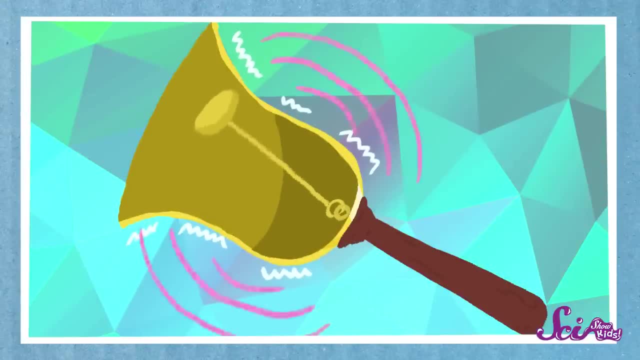 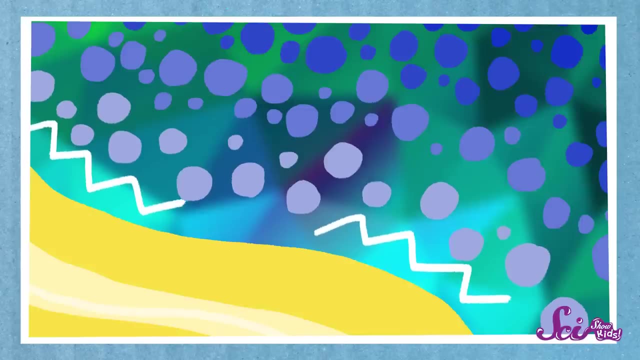 the metal that makes up the bell to vibrate really fast back and forth, And the vibration of the bell also shakes up the particles that make up the air around it and makes them vibrate. Then those particles run into the air particles next to them and so on. You can also think about it like: 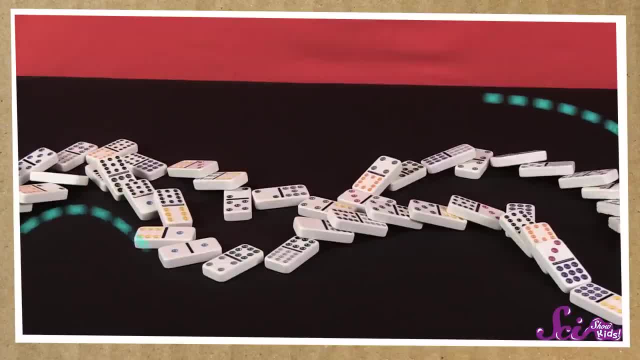 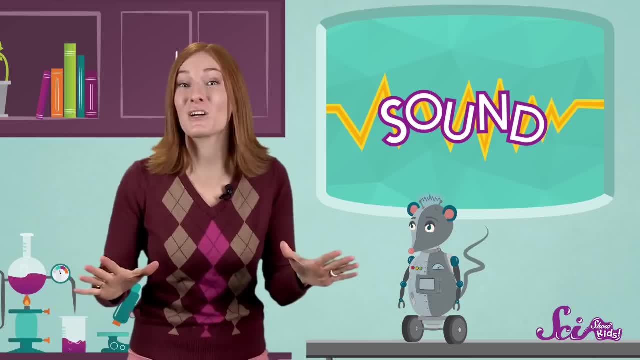 dominoes, with the vibration getting passed along from one bunch of particles to the other particles in the air to the next. We call this path of vibration a wave. Now how do we hear those vibrations? If we could look deep inside our ears we'd see.